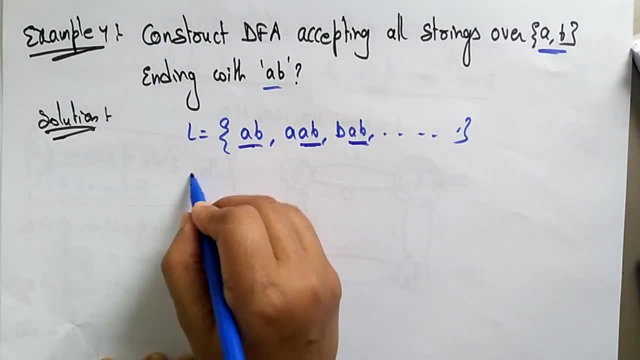 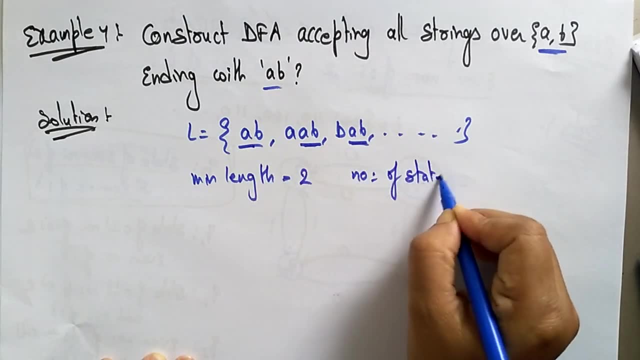 should be A, B. So what is the minimum length here? The minimum length is 2.. So number of states so participating in the DFA, or the number of states is equal to 2 plus 1, 3 states are there. 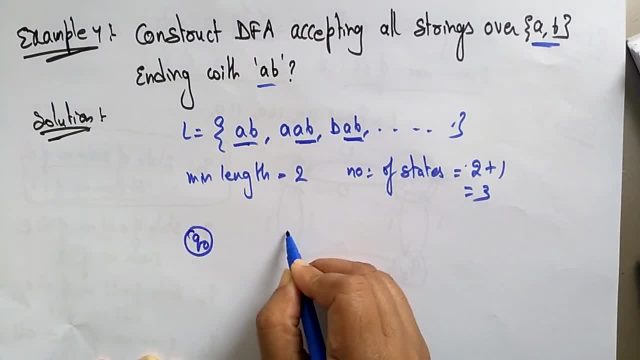 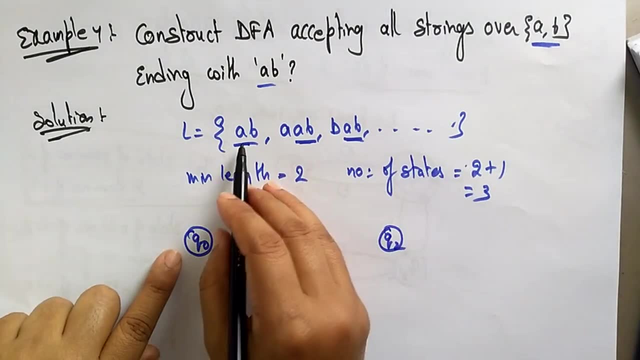 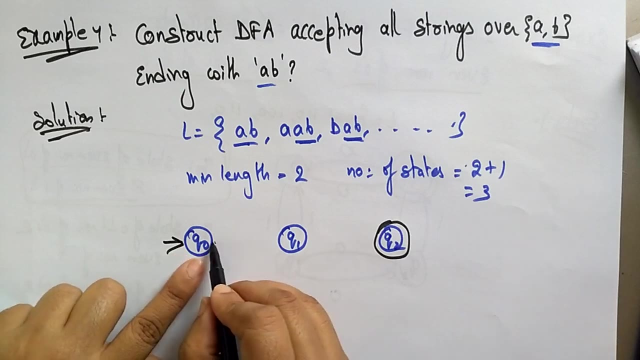 Okay, So let me take Q. naught Q1 and Q2.. Okay, So first take the minimum length. This is the initial state and let me take. this is the final state. Why I am taking this final state means C. 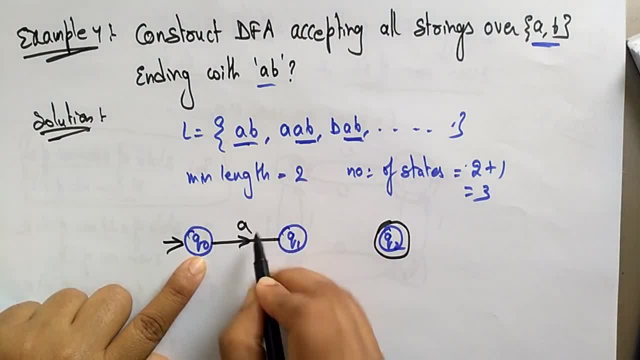 here. So if you take minimum length, Q naught on A goes to Q1, and Q naught on B goes to Q2.. So the A- B string is accepted because it has to reach the final state. So Q naught on A goes to Q1, which is a transition function. next state: Q1 on B transition. 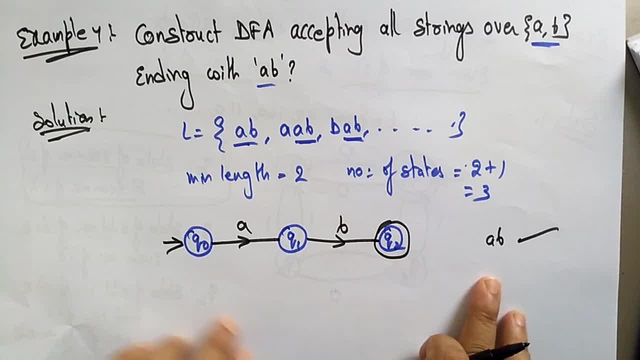 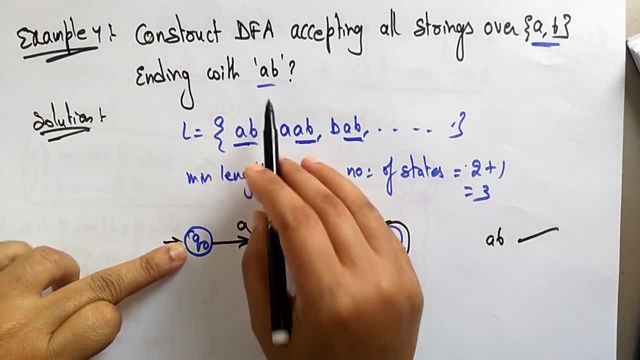 function leads to final state Q2.. So A, B is accepted. Okay, So Q naught the string should starts with the. they didn't say that string has starts with either A or B. it doesn't say anything. 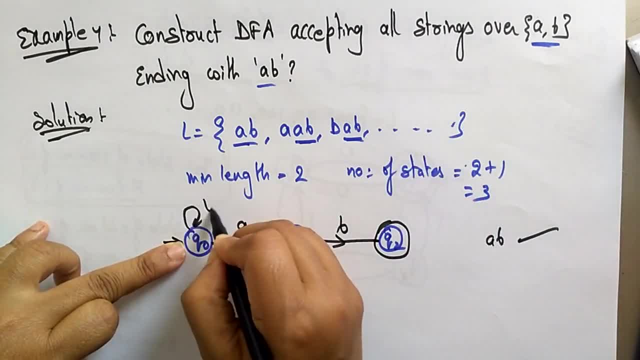 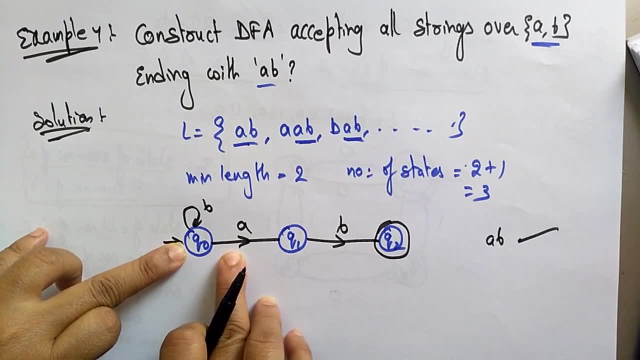 So it can be start with A or it can start with the B. Okay, So the Q naught can start with A, that is also true, and the Q naught can start with B. this is also true. So because it is B, So B, A, B is. 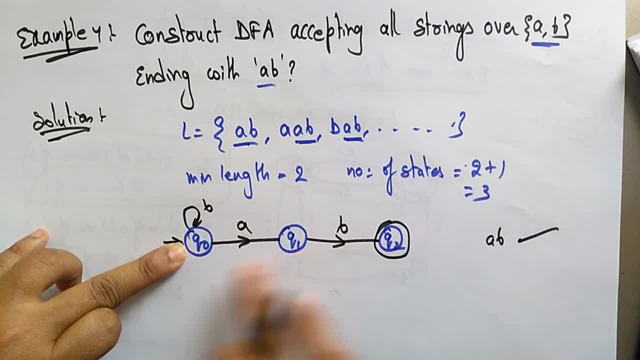 accepted. Okay, A, B is also accepted. So now coming to the Q1.. So the Q1 is: first it's going to the B and next input is A should be there. So the final is it has to reach to the B, B, A. 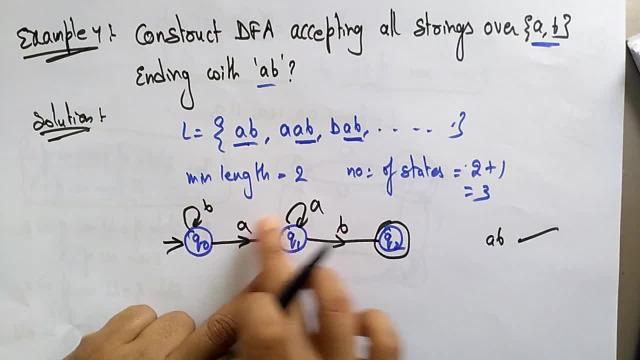 A B. So the ending of the string should be A only. So B, A, A, B. So this is also accepted Because the ending should be A, B. So Q1 is over, Now coming to the Q2.. So Q2,, Q2, the string. 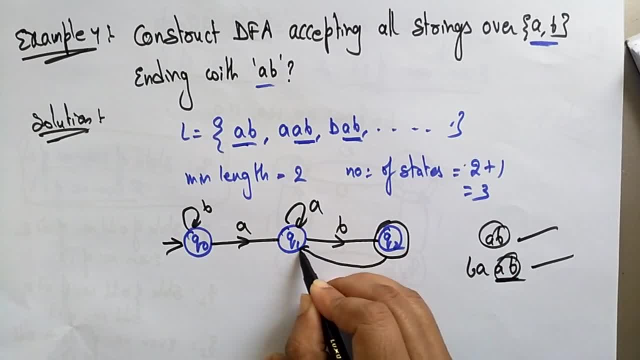 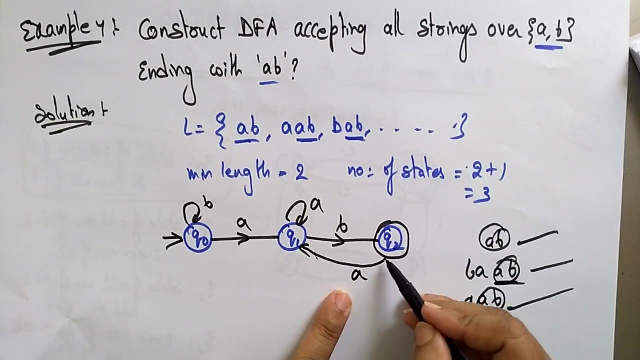 should end with A, B So A. if I take this, if I take Q2 on A, it goes to A. on Q1, A, it goes to A, A B, So A, A, A B. So this is also accepted. So that's why I have taken the input A Next. 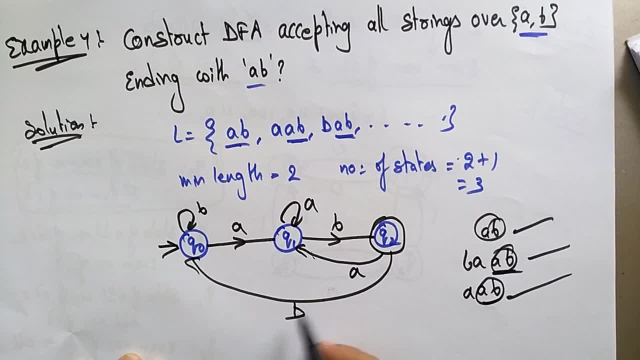 the input on B, So Q2 on B, B, B, A, A, B. Okay Means, whatever the intermediate you are taking, the final should be end with A, B. So that's why I have constructed this DFA. You will get a doubt. 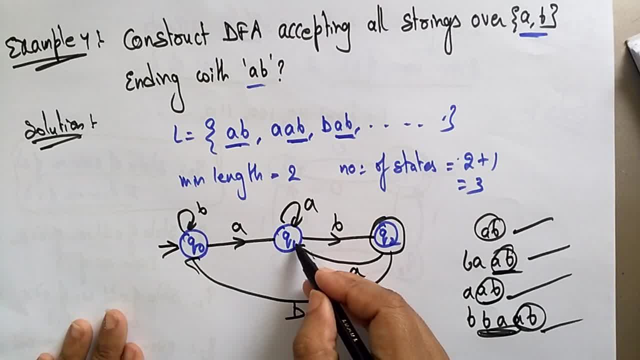 how you understand, how can I know that I have go to A like this and I have go to B for here, only not here, Because in the DFA there is a rule: only one path should be there for one state. So 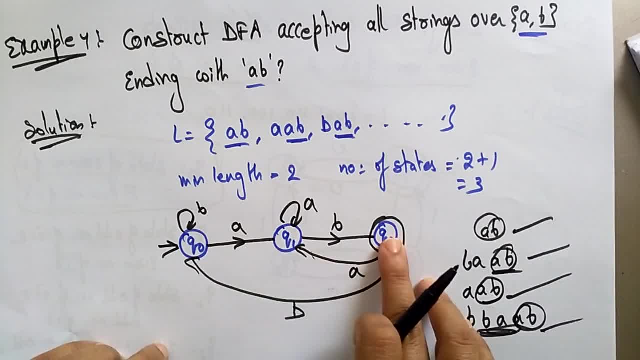 for one state it has to go only one input: A- Okay, Here you can't go. the B cannot goes to here. Okay, Suppose, if I take the B loop here, I will get BB, BB. So the BB string is not accepted. 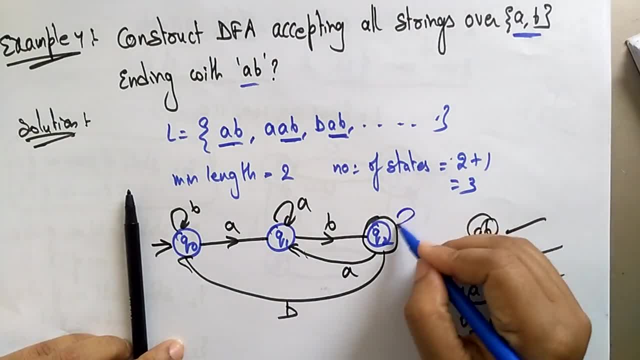 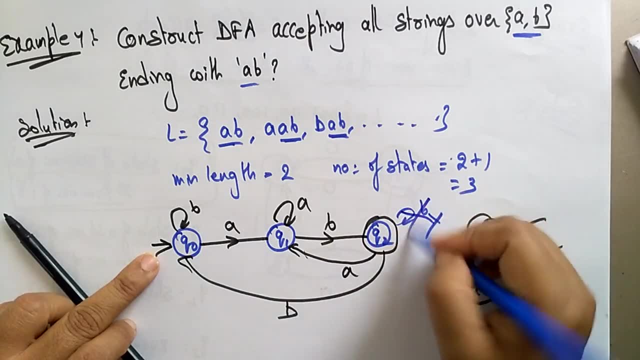 Suppose if I take in something like here, if I, you will get it. or suppose if I take here, this is wrong Because B, A, A, BB, the string will ends with the BB. but it is wrong, So that's why I have taken the loop to here. I can't take to here. 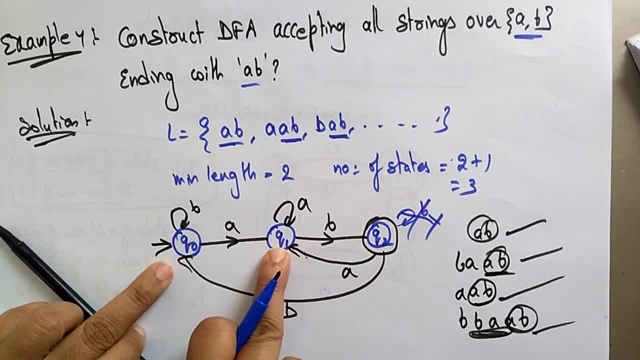 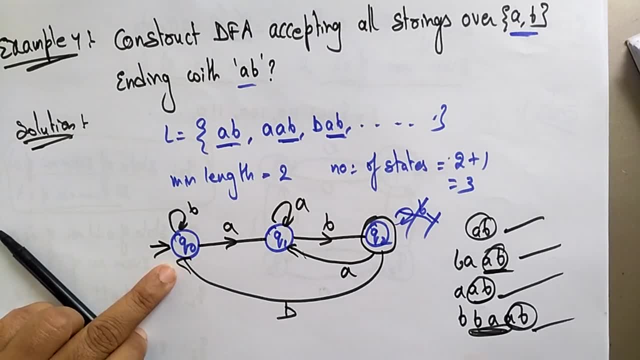 because already Q2 is going to next state on A to Q1.. So next in the DFA I have to choose another state on that, another input, because only one path should be there for one input. Okay, So this is the DFA. accept all strings over AB. So don't be confused. If you know the rules, then you can. 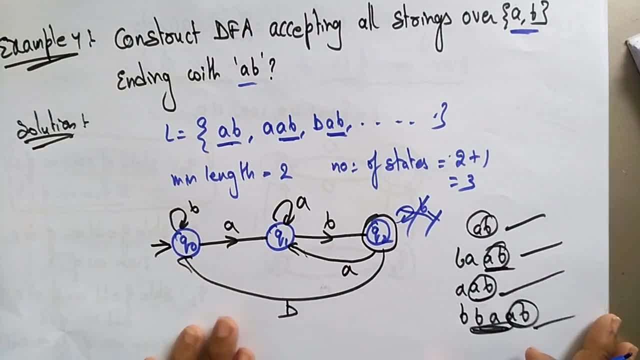 easily construct. by seeing this question, you can easily construct that state. Okay, Thank you. 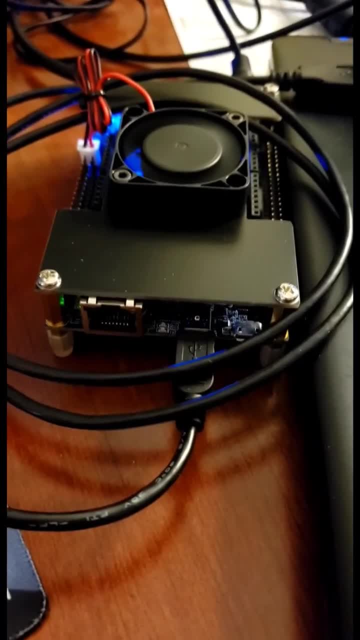 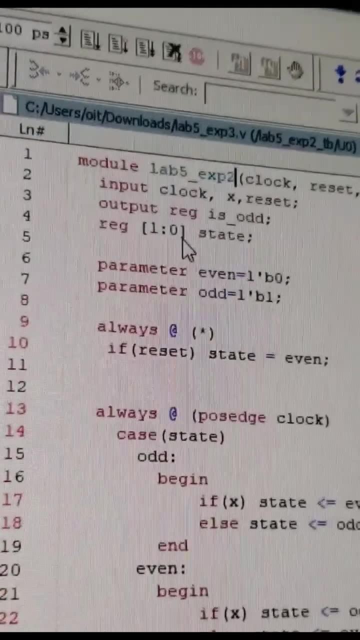 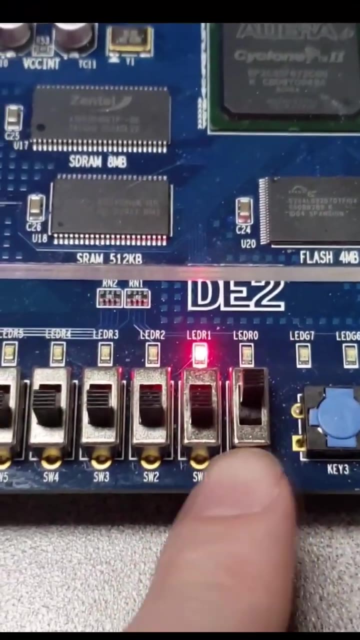 Want to design custom circuits for an FPGA? Here's how. Capture your design using a hardware description language like VHDL or Verilog. Verify your design by simulating its behavior. Synthesize your code into a netlist Place and route the netlist to determine physical locations of logic elements.